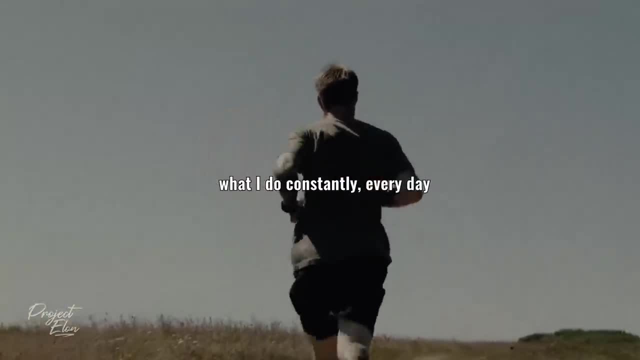 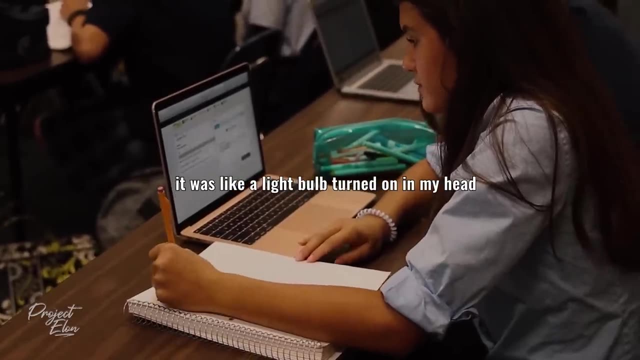 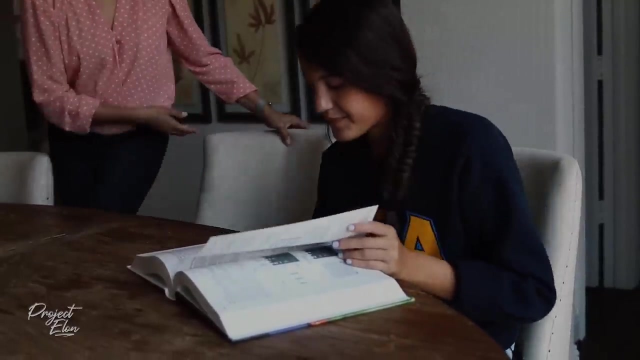 I realized it came down to my daily habits. What I do constantly, every day, will determine what grades I achieve. It was like a light bulb turned on in my head. What I do with my 24 hours will determine whether I succeed or fail. Those that perform in the top 1% when they don't feel like studying, they do it anyway. 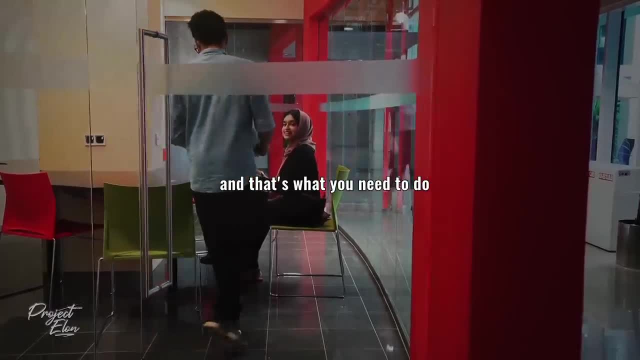 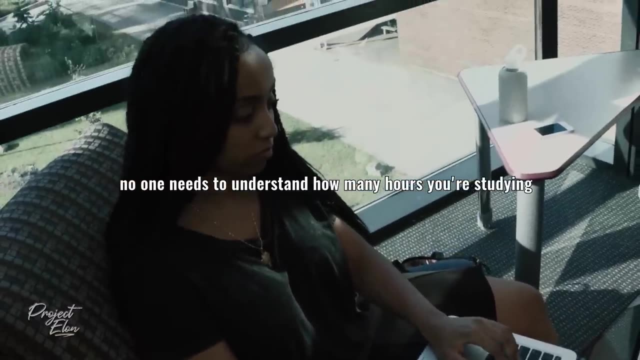 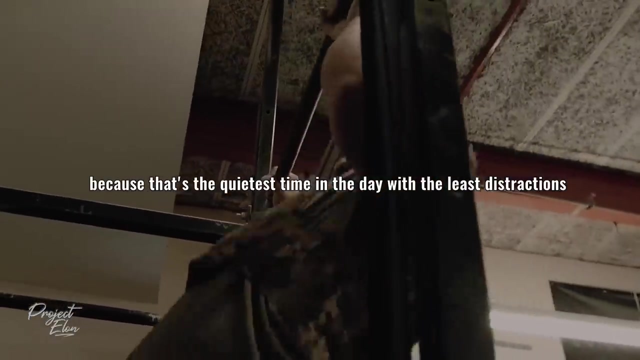 And that's what I started to do, And that's what you need to do. You study hard even when no one is watching. No one needs to understand how many hours you're studying. No one needs to know how early you wake up in the morning, because that's the quietest time in the day, with the least distractions. 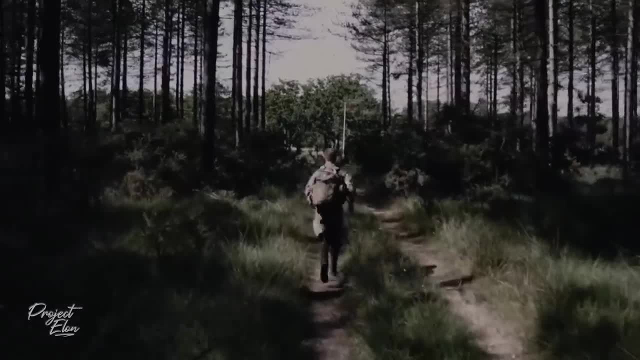 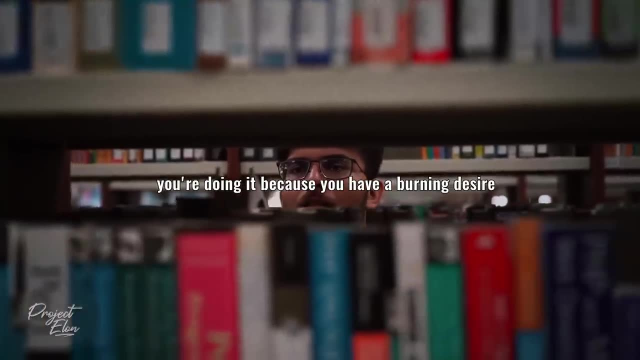 No one even needs to know why you're studying. No one needs to know how many hours you're studying. You're not doing it because of the grades or to prove to the people around you that you can do it. You're doing it because you have a burning desire: Step by step, day by day, become the best. 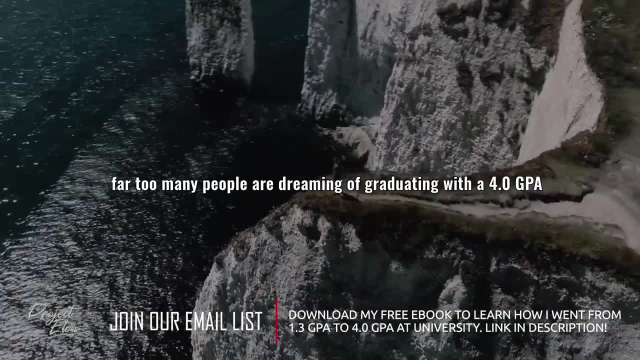 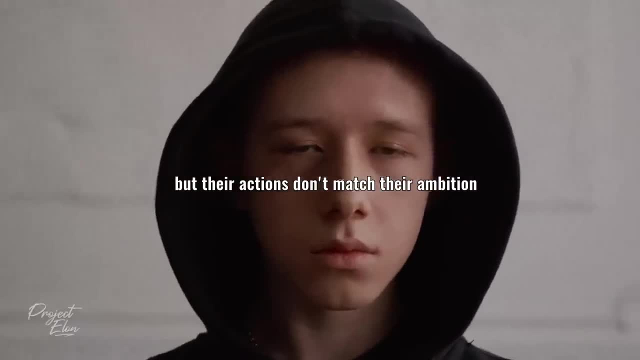 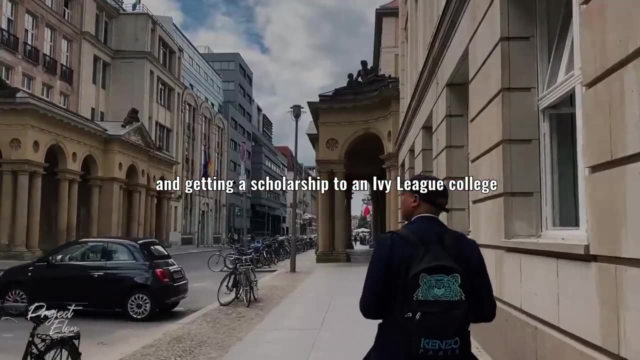 version of yourself possible. Far too many people are dreaming of graduating with a 4.0 GPA, But their actions don't match their ambition. They're dreaming of graduating at the top of their life. They're dreaming of becoming top of their class and getting a scholarship to an Ivy League college. 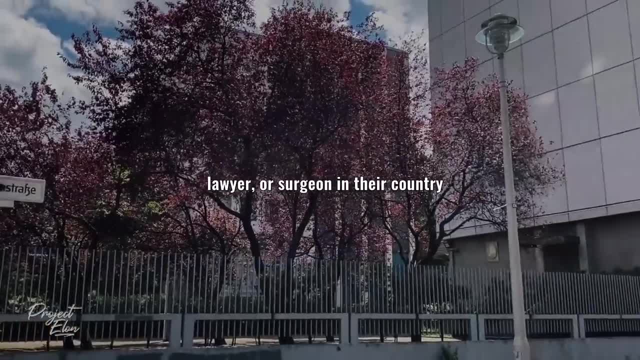 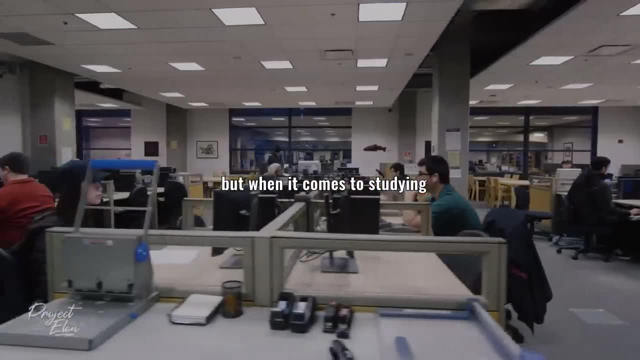 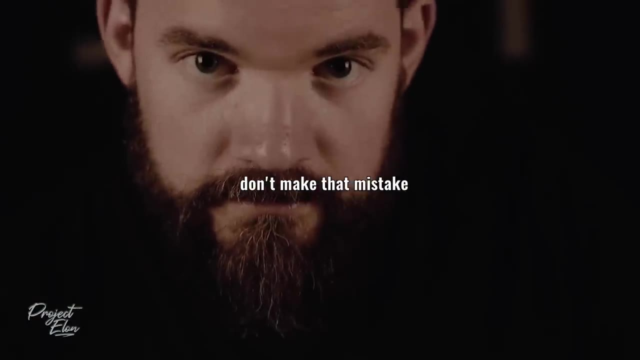 They're dreaming of being the best doctor, lawyer or surgeon in their country. They're dreaming of buying a huge house and a fast car, But when it comes to studying, they can't last 30 minutes without getting distracted. Don't make that mistake. 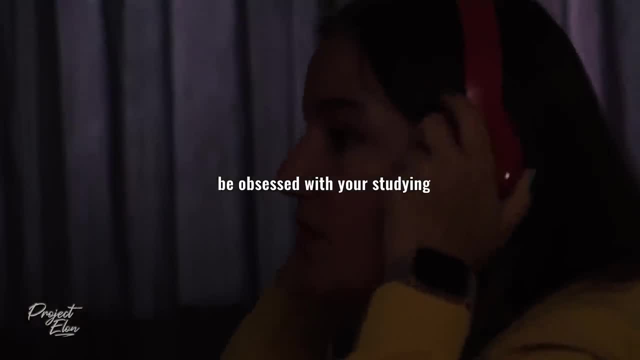 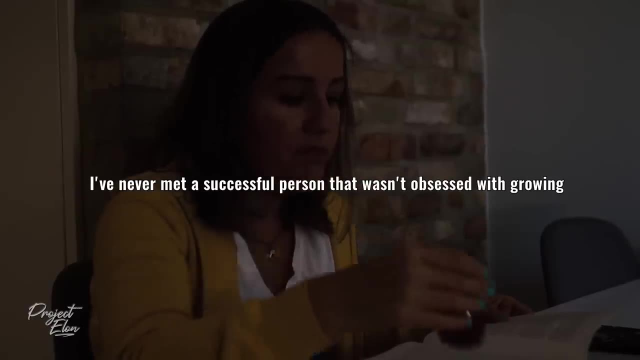 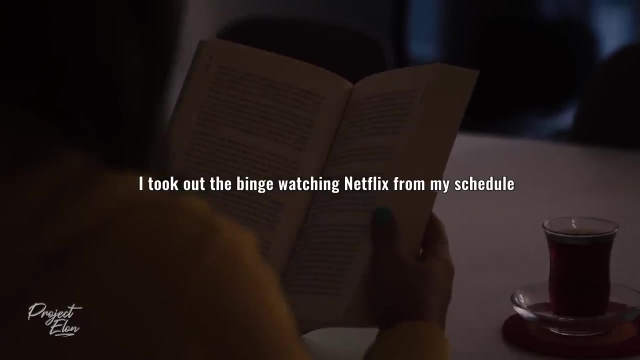 Let your actions do the talking. Be obsessed with your studying, with learning, with growing up, with learning, with learning, with learning. I've never met a successful person that wasn't obsessed with growing. That's what I did: I took out the binge-watching Netflix from my schedule and replaced it with personal development. 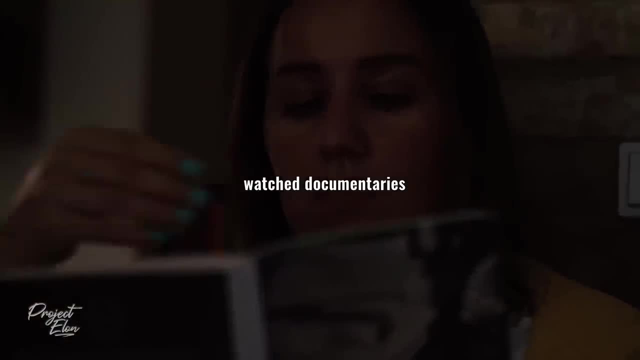 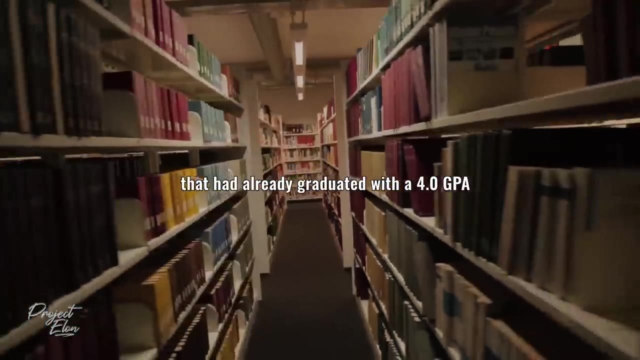 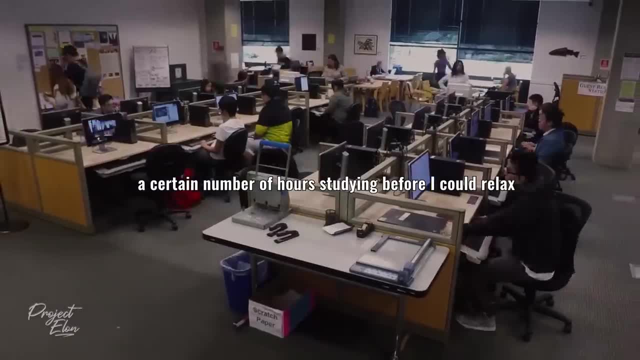 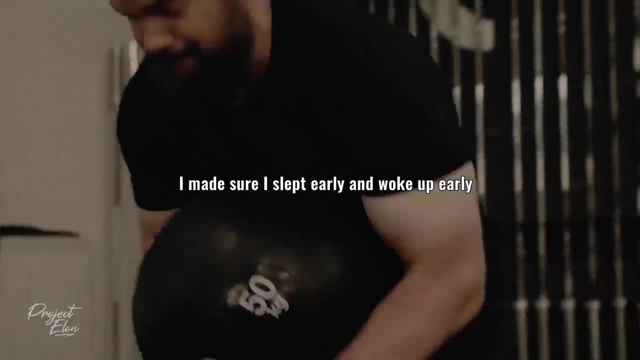 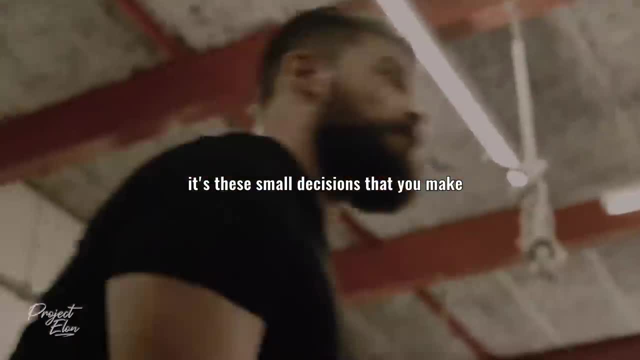 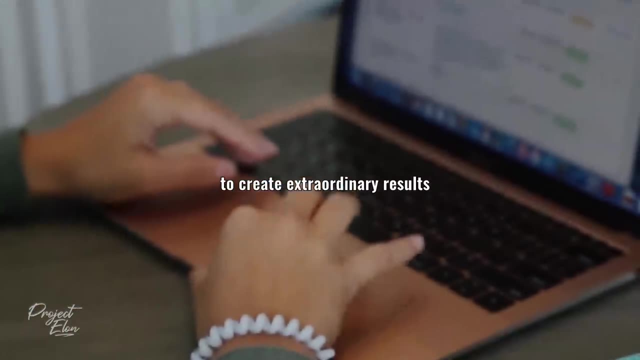 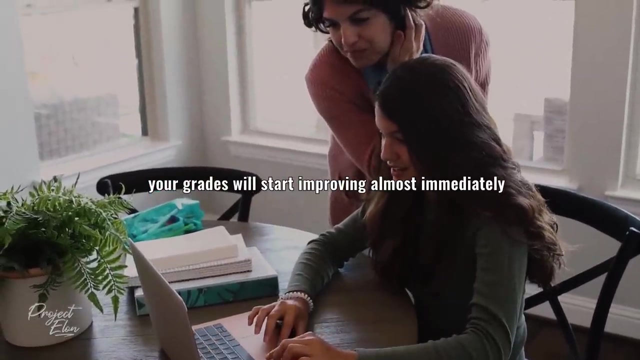 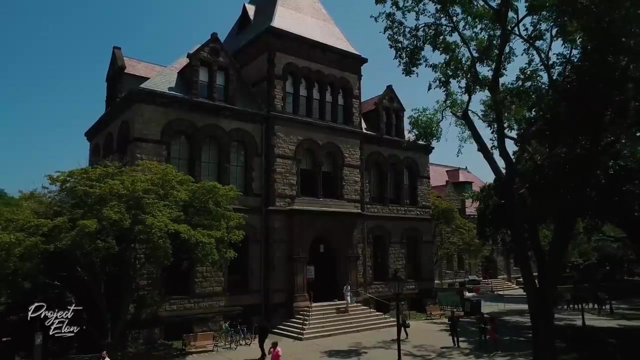 It's these small decisions that you make, The seemingly insignificant decisions that build up over time to create extraordinary results. After a few weeks you will start to see results. Your grades will start improving almost immediately. You will start feeling better about yourself, happier, more content with your life. 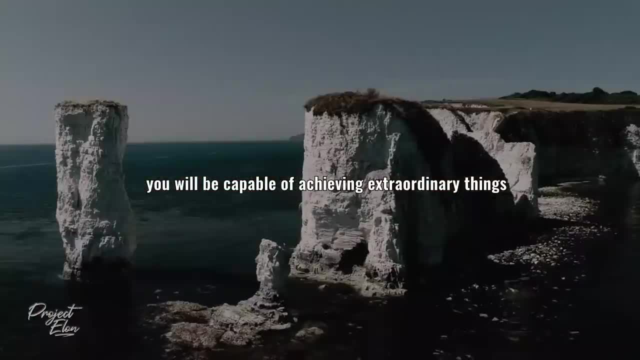 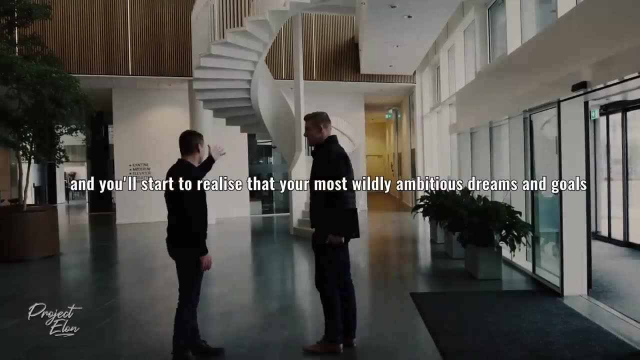 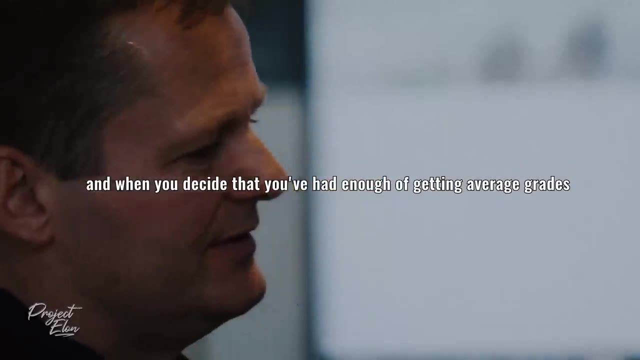 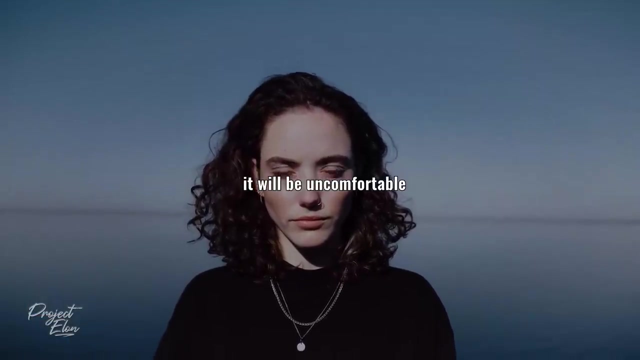 And after years of living like this, you will be capable of achieving extraordinary things And you'll start to realize that your most wildly ambitious dreams and goals actually start becoming achievable. And when you decide that you've had enough of getting average grades, just like I did, let me warn you: it will be painful And it will be uncomfortable. 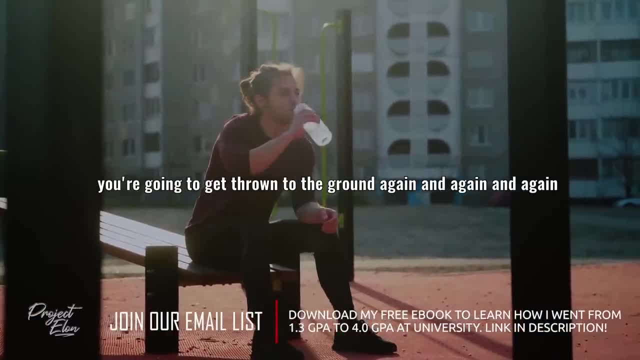 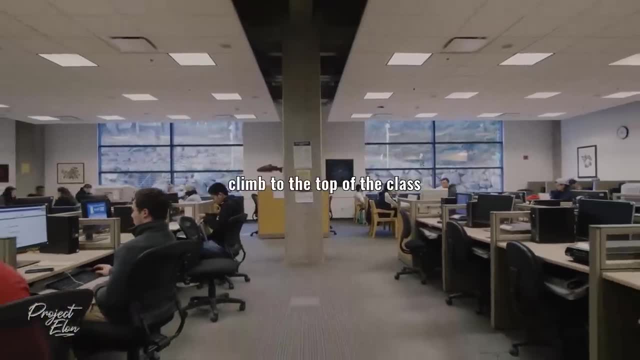 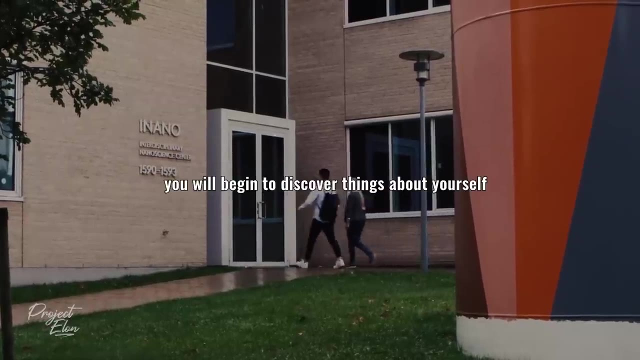 But that's where the growth is. You're going to get thrown to the ground again and again and again. But when you have the determination to climb to the top of the class and when you know that what you're doing, by studying every day, will be rewarded, you will begin. 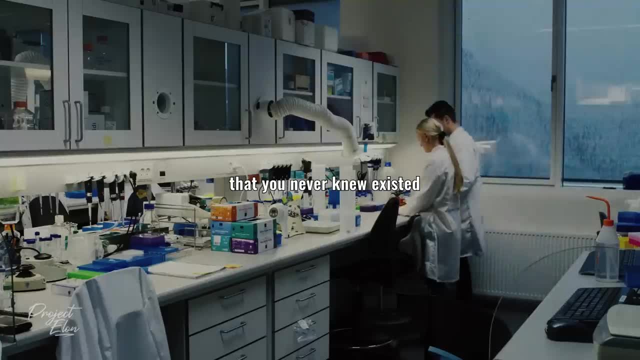 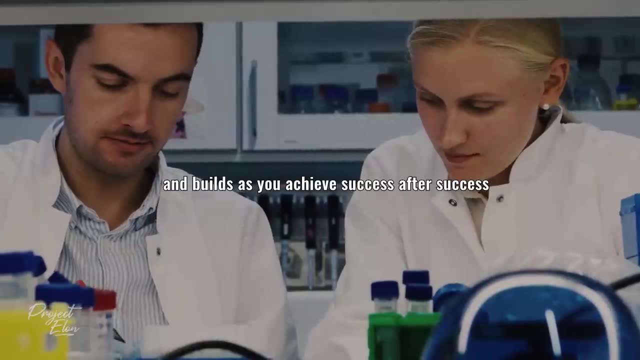 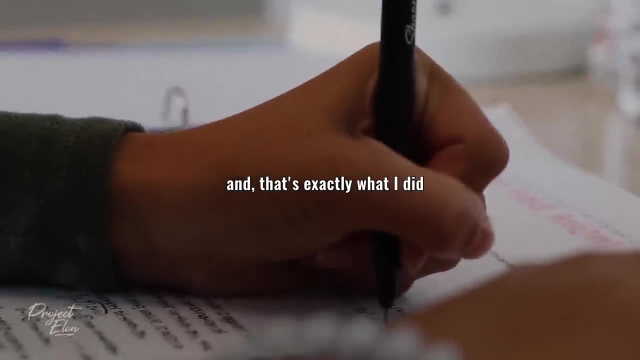 to discover things about yourself that you never knew you could … exists and will help you work towards your goals. You will have an energy that just builds and builds as you achieve success after success. And that's exactly what I did, And if I did it, you can too. Look, I got rid of the 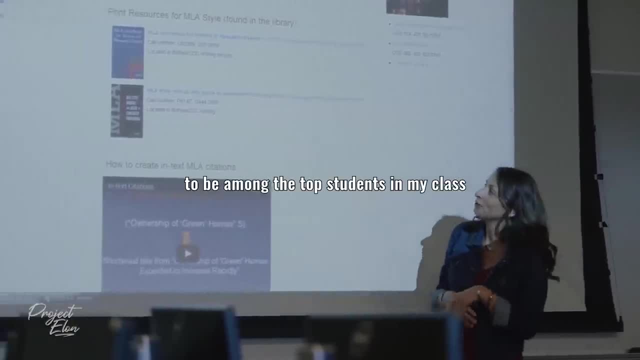 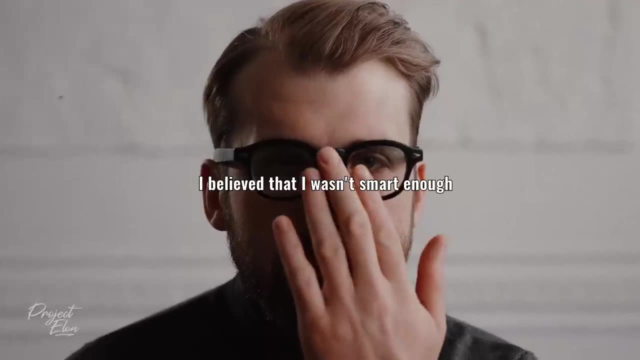 mindset that I'm not smart enough to be among the top students in my class. It was a self-fulfilling prophecy that I was stuck in for a long time. I believed that I wasn't smart enough, And so my grades reflected that. 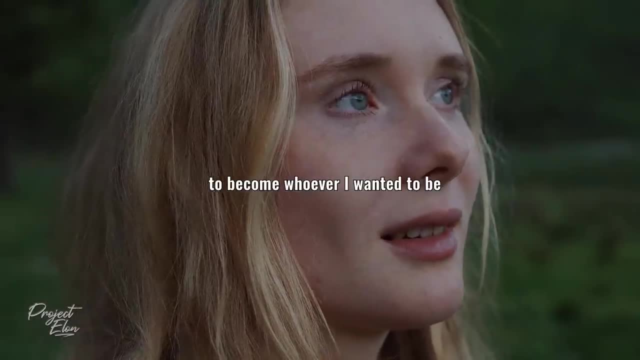 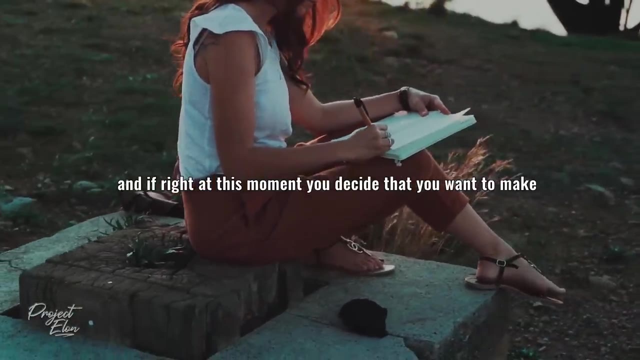 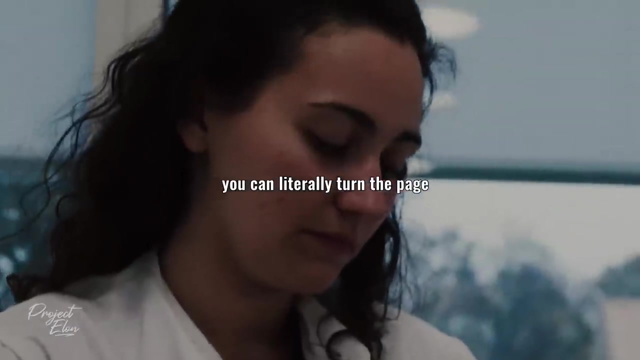 Once I threw away that mindset, it freed me to become whoever I wanted to be. You write your own book And if, right at this moment, you decide that you want to make this a new chapter, you can literally turn the page in your life.